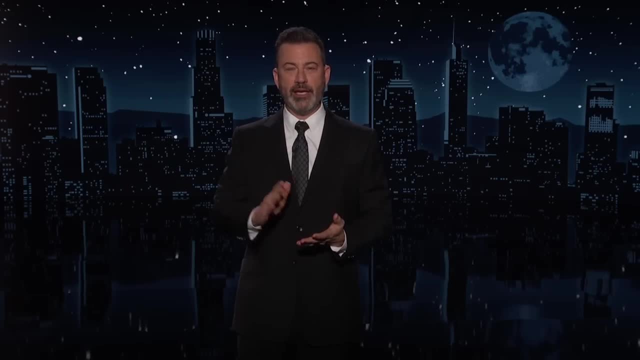 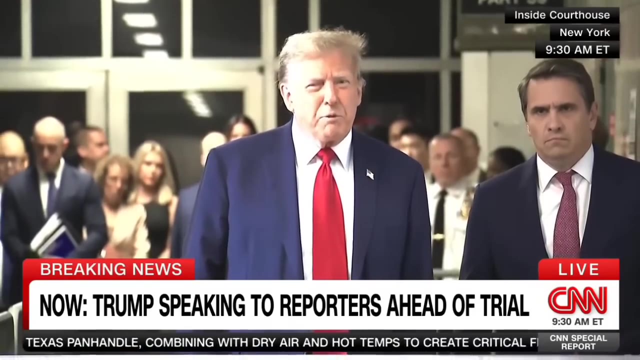 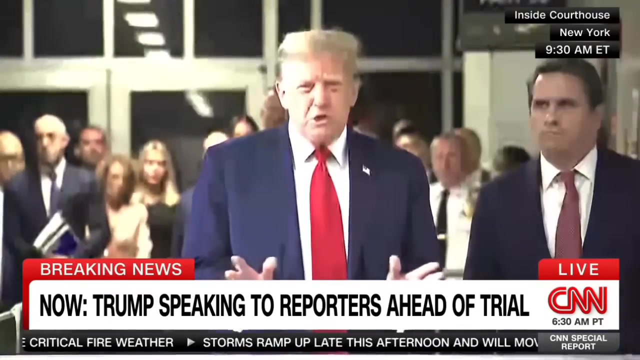 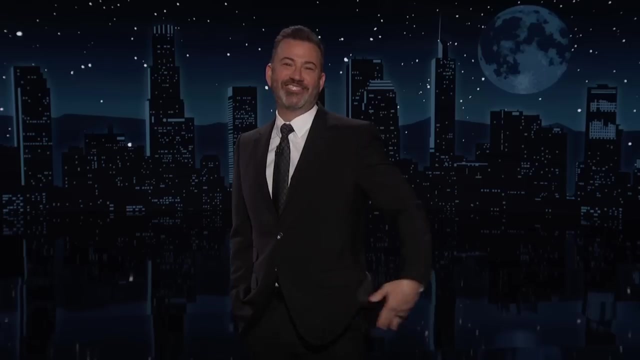 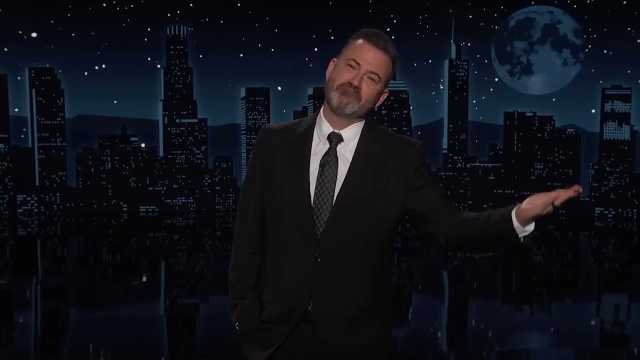 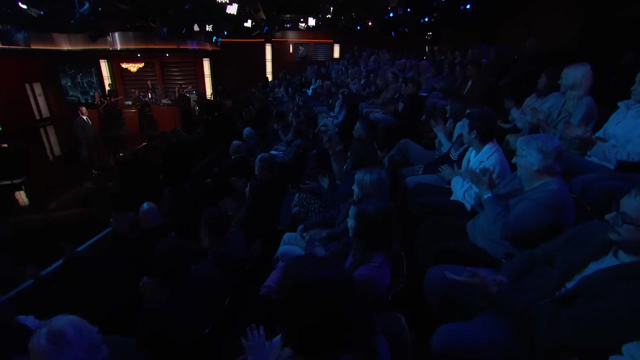 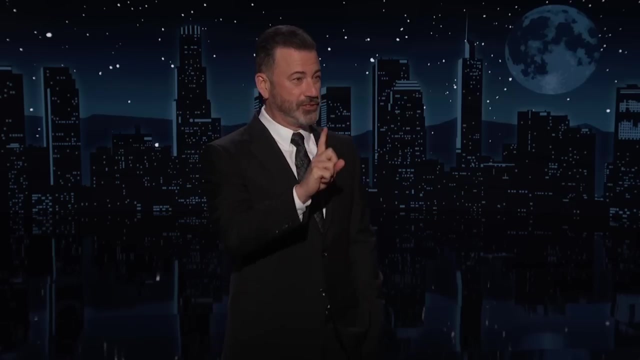 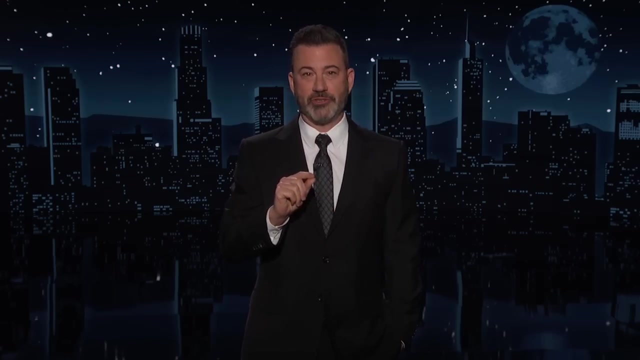 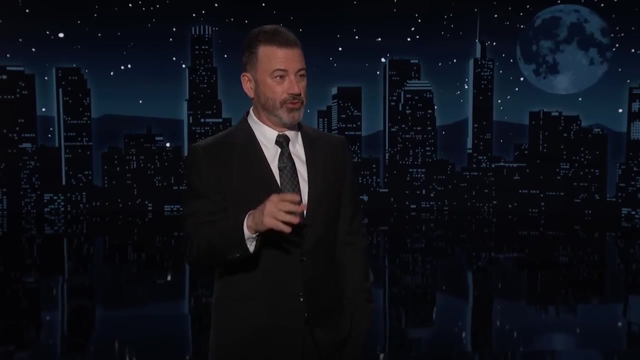 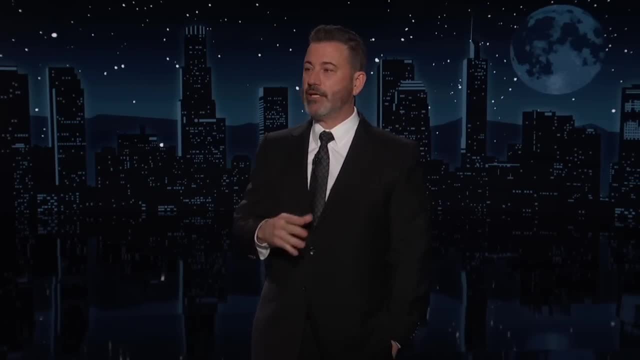 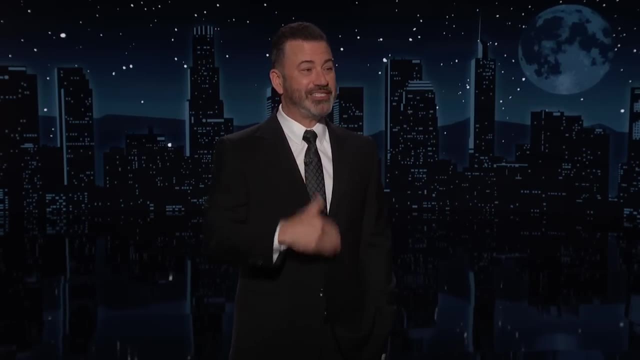 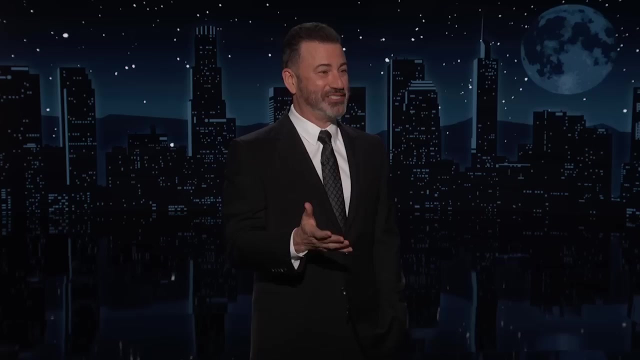 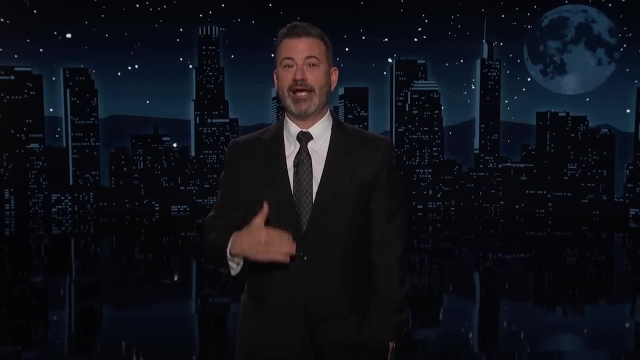 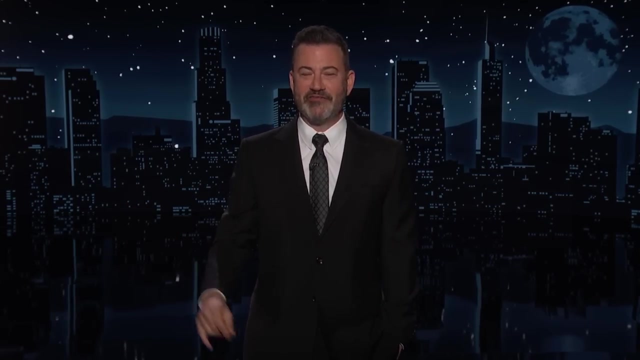 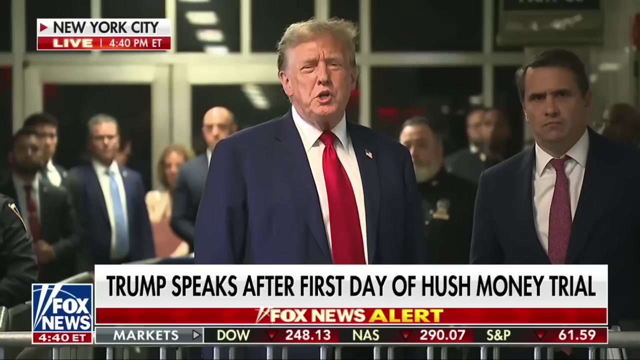 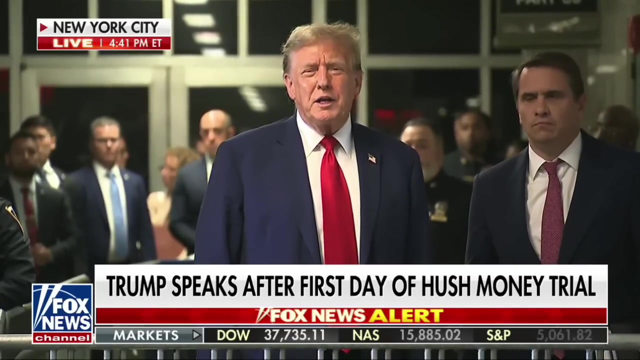 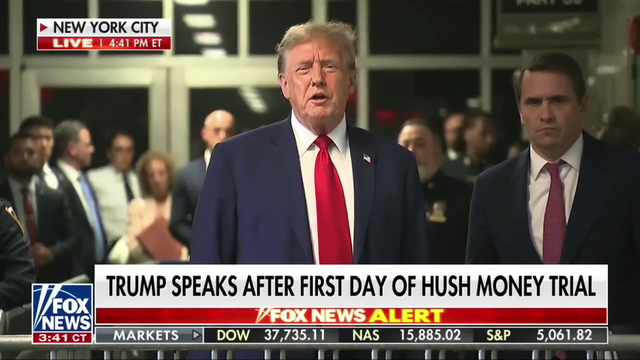 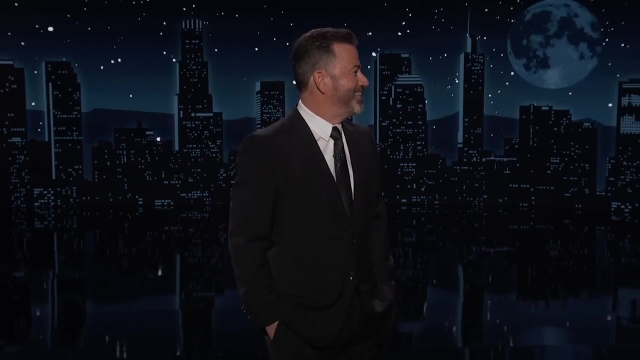 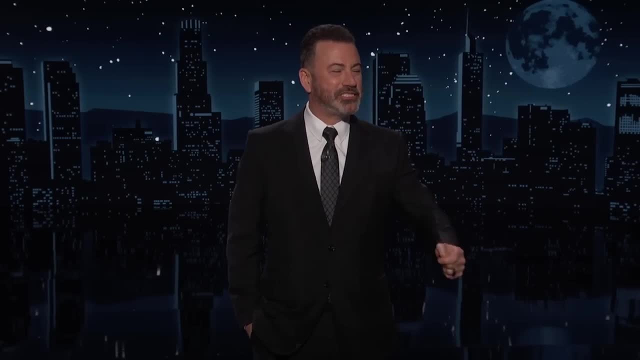 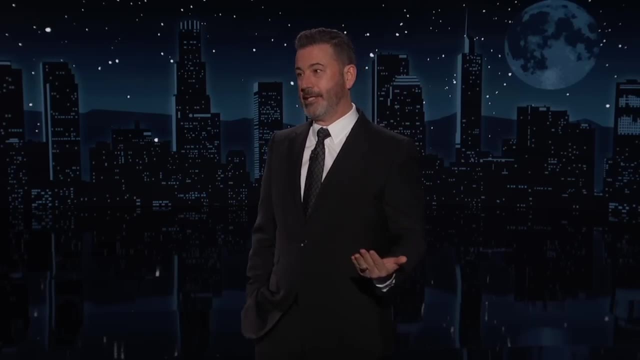 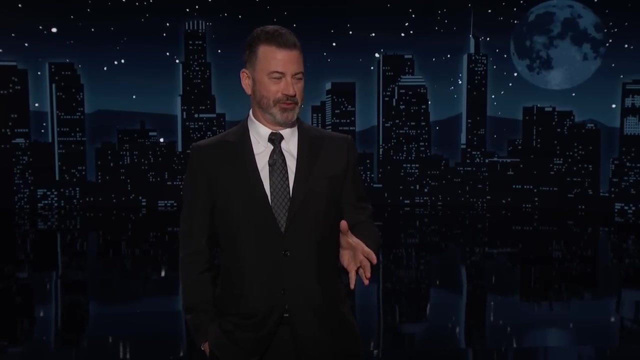 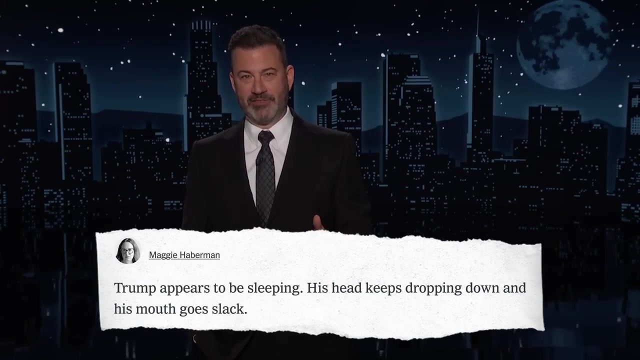 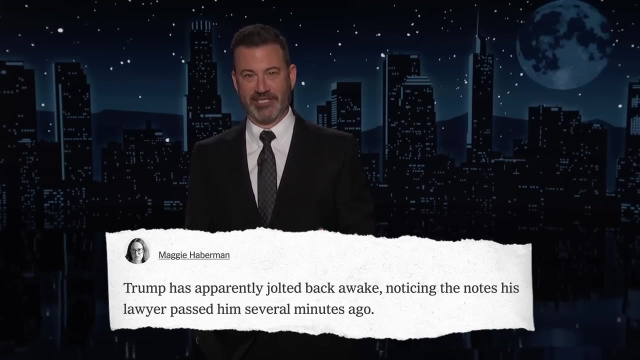 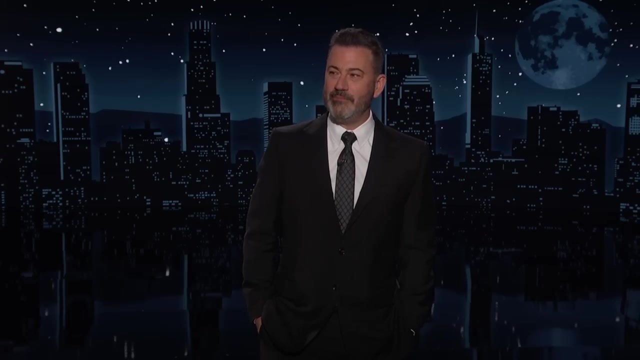 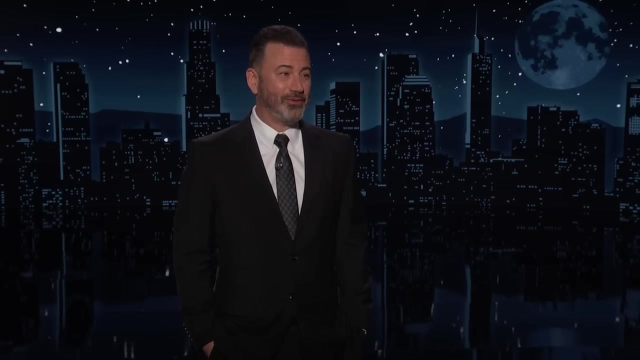 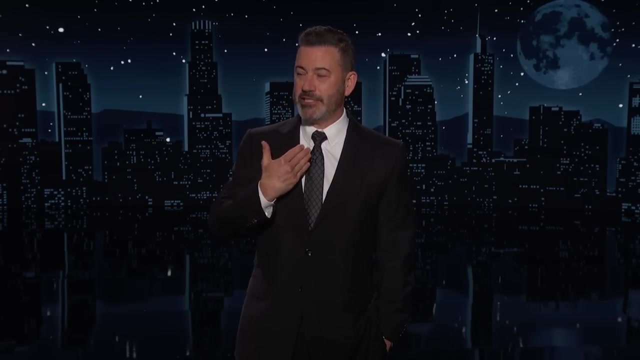 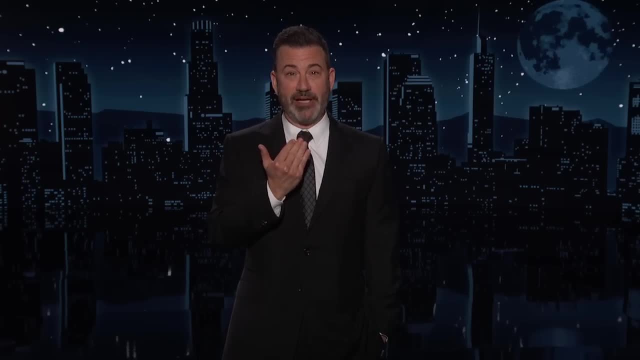 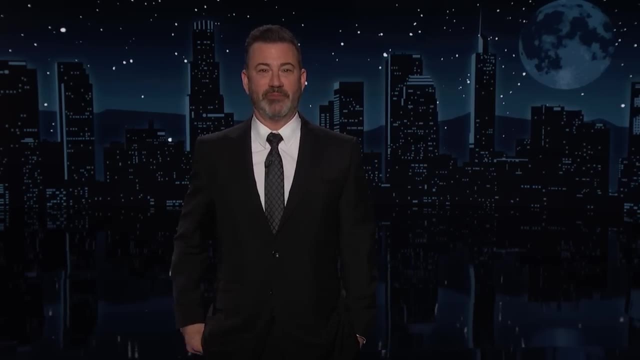 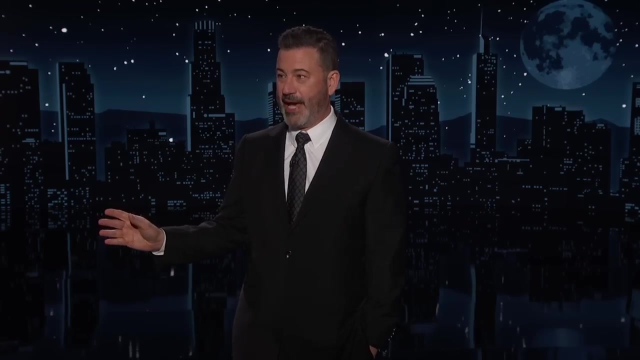 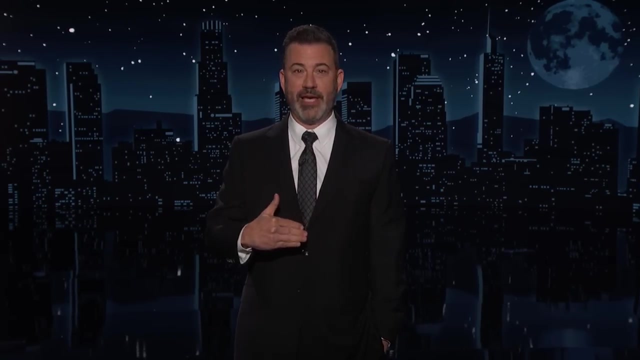 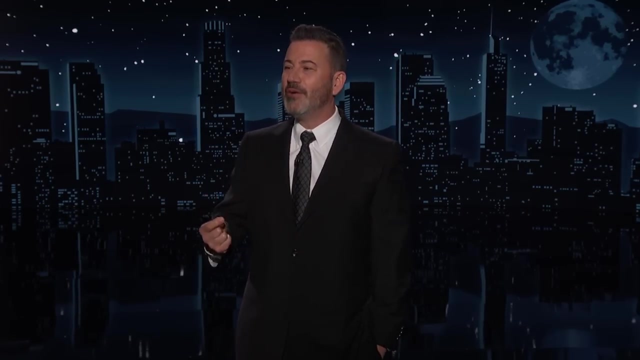 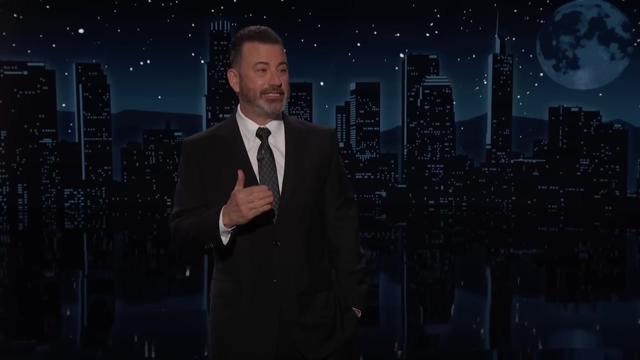 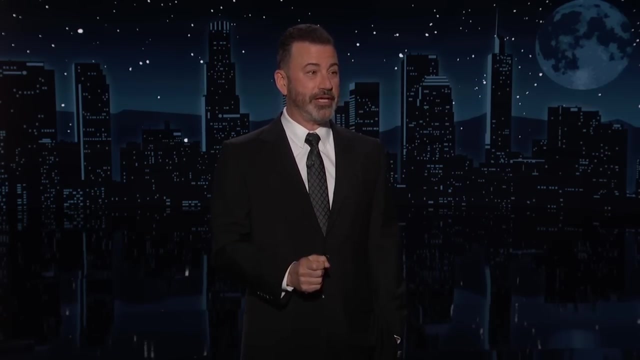 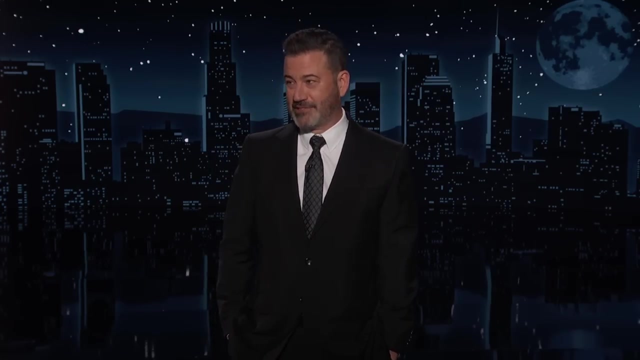 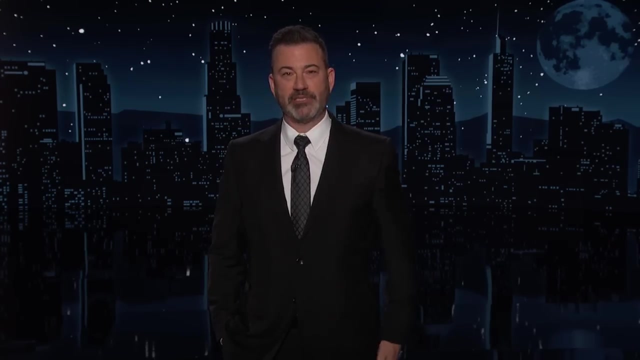 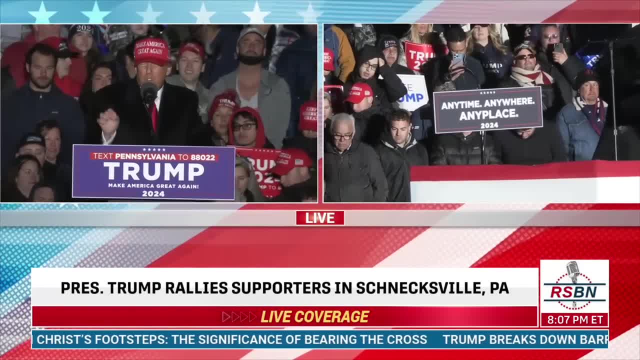 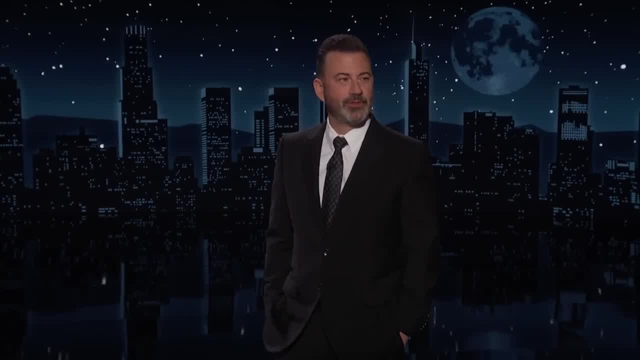 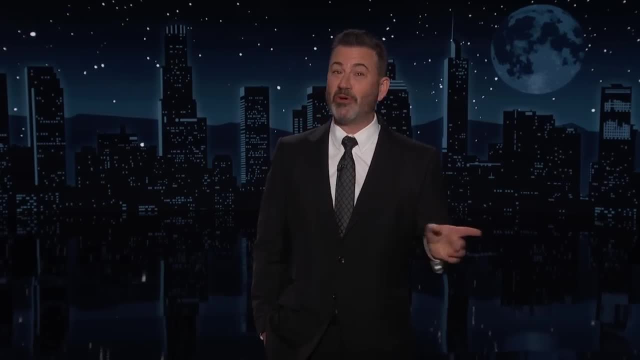 Just four years ago was the exact opposite. We were the most respected country in the world. We were the most respected that we were ever respected. Out of all the respect that had ever been respected, we were the most respected back then, And that wasn't even close to the court of the night. 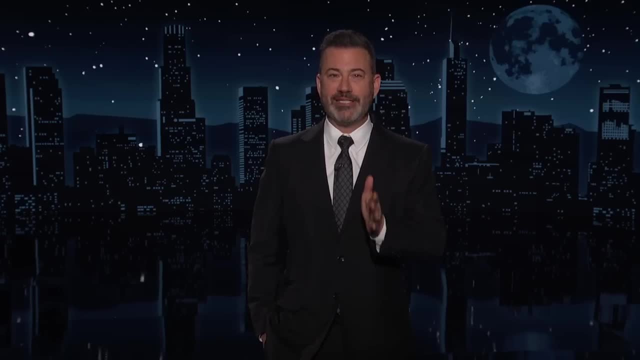 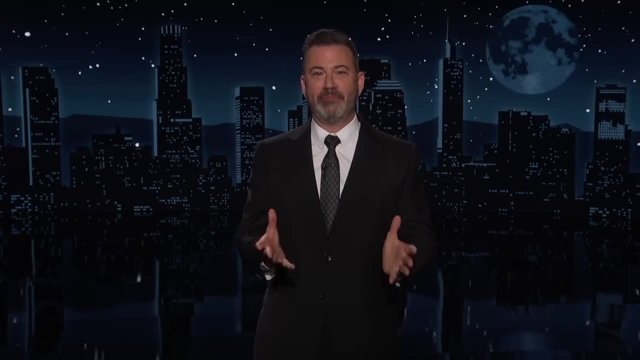 You have to hand it to this guy On the weekend before his unprecedented criminal trial begins. he somehow manages to overshadow it with this broken-brained interpretation of what happened at Gettysburg during the Civil War. Buckle up everybody. This is an all-timer. 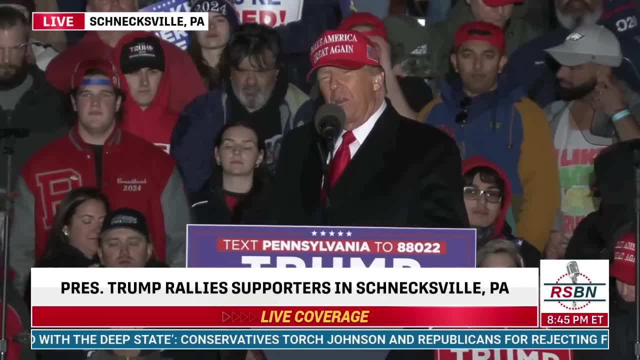 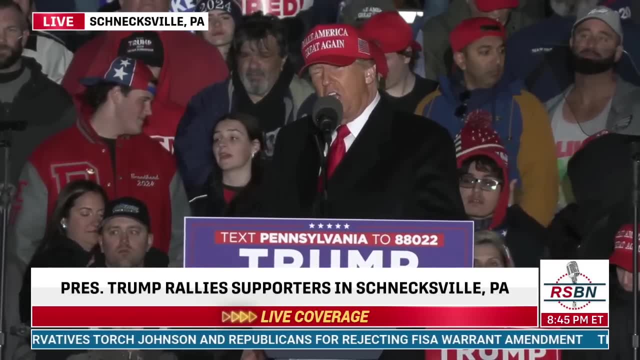 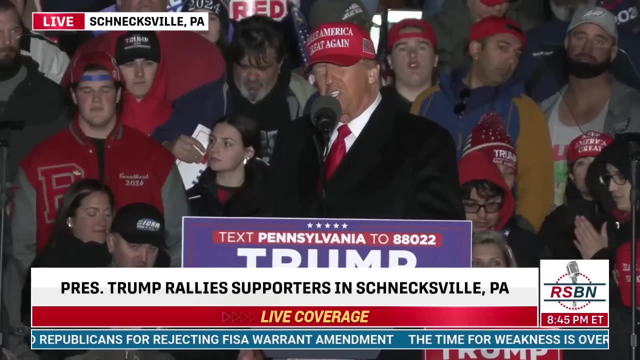 Gettysburg. what an unbelievable battle that was The Battle of Gettysburg. what an unbelievable, I mean. it was so much and so interesting and so vicious and horrible and so beautiful in so many different ways. It represented such a big portion of the success of this country. 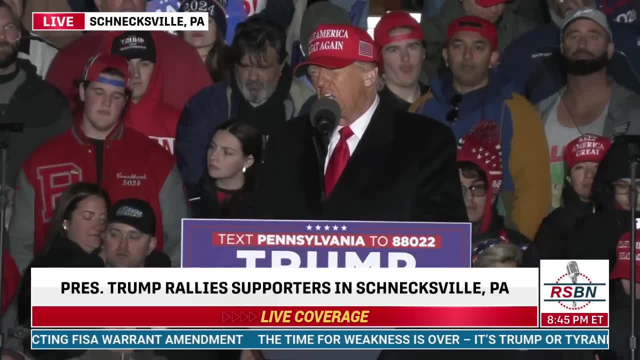 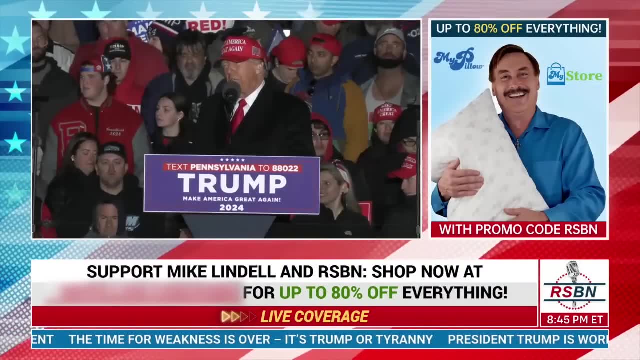 Gettysburg- wow, I go to Gettysburg, Pennsylvania, to look and to watch, and And the statement of Robert E Lee, who's no longer in favor. Did you ever notice that? No longer in favor. 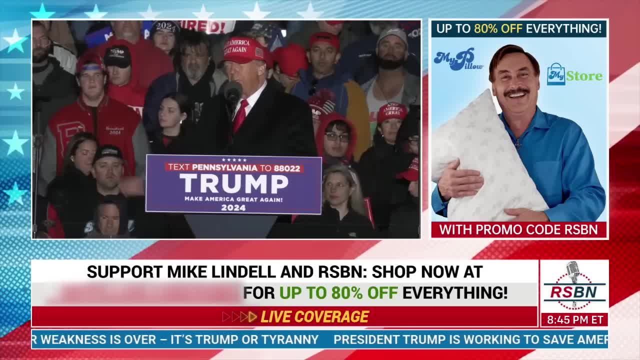 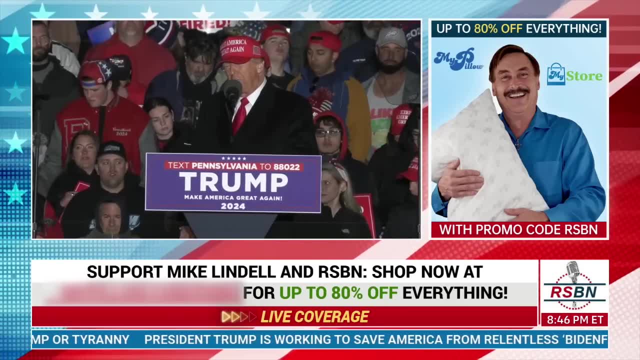 Never fight uphill me boys, Never fight uphill. They were fighting uphill. He said: wow, that was a big mistake, He lost his great general And they were fighting: Never fight uphill me boys. But it was too late. 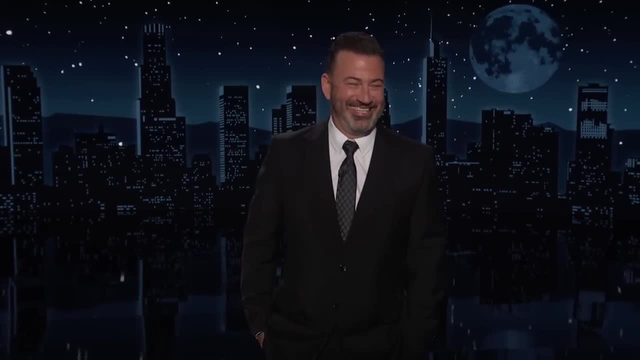 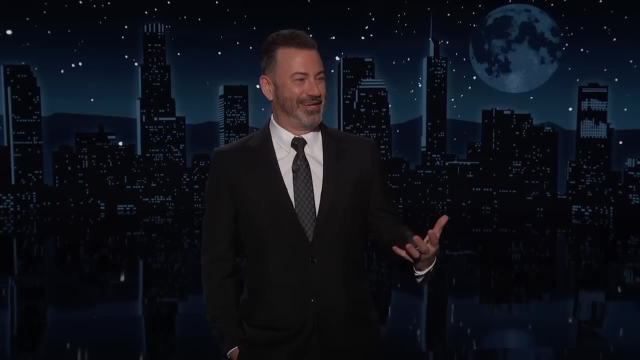 No, I don't know. That was easily the funniest seizure I've ever seen. He always sounds like a kid who forgot he had an oral report due on that day. More than 50,000 Americans killed each other over three days at Gettysburg. 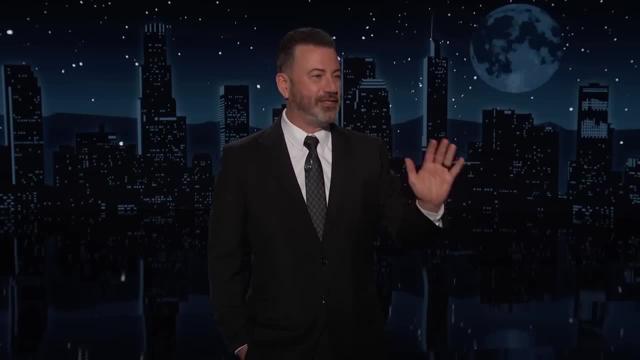 so I'm not exactly sure what he meant by beautiful, But let's give him the benefit of the doubt and let's go through his actual words. Guillermo, bring out the chalkboard if you would. Now we have a transcript. 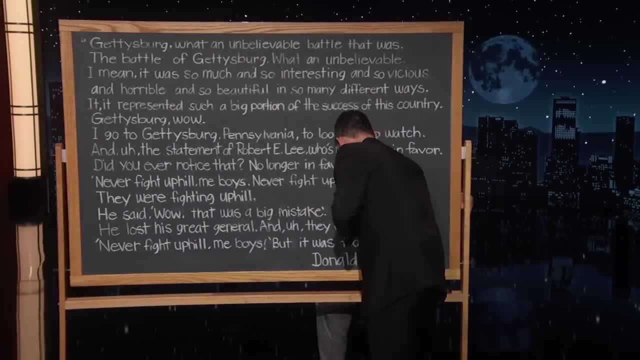 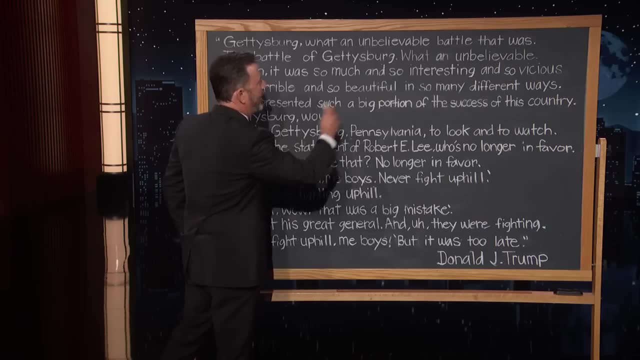 of what our former president said And I'll just go through it. Thank you, Guillermo, You're welcome, man. Here we go. Gettysburg- What an unbelievable battle That was The Battle of Gettysburg. 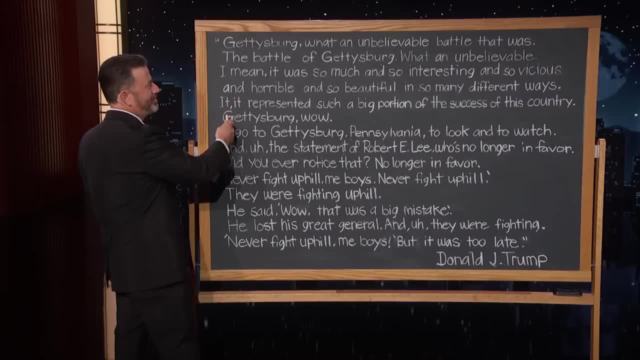 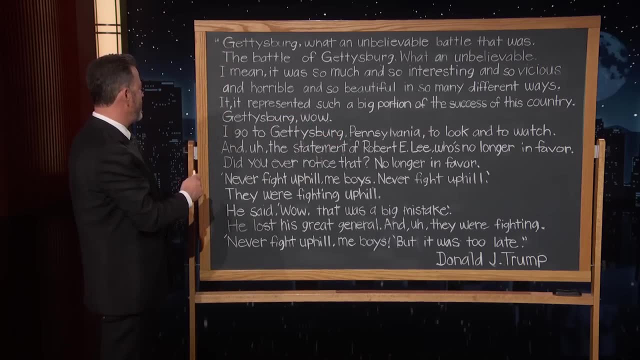 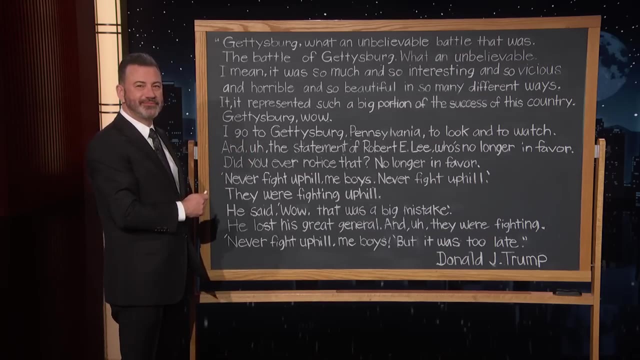 What an unbelievable. I mean it was so much and so interesting and so vicious and horrible and so beautiful in so many different ways. It represented such a big portion of the success of this country. Gettysburg- Wow, I go to Gettysburg, Pennsylvania. 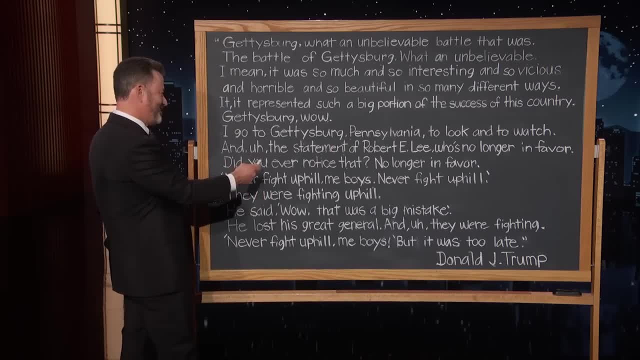 to look and to watch, And the statement of Robert E Lee, who's no longer in favor. did you ever notice that? No longer in favor? Never fight uphill, me boys, Never fight uphill. They were fighting uphill. He said: wow, that was a big mistake. 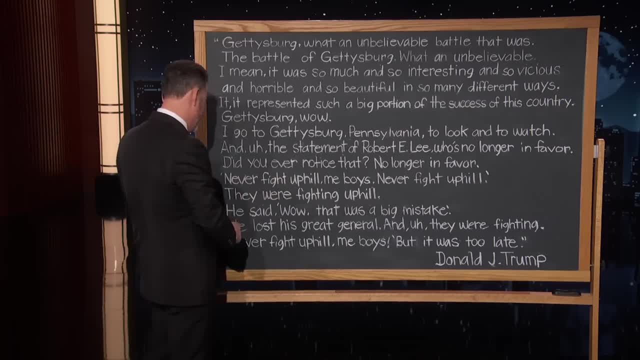 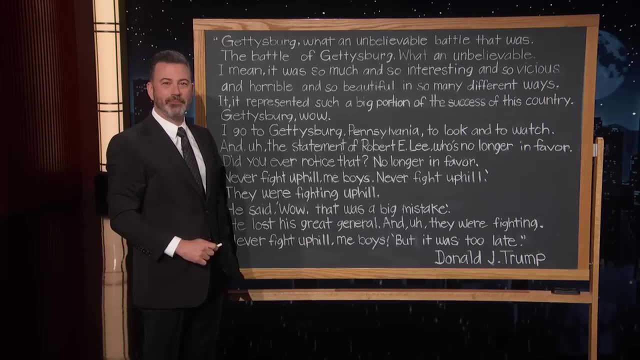 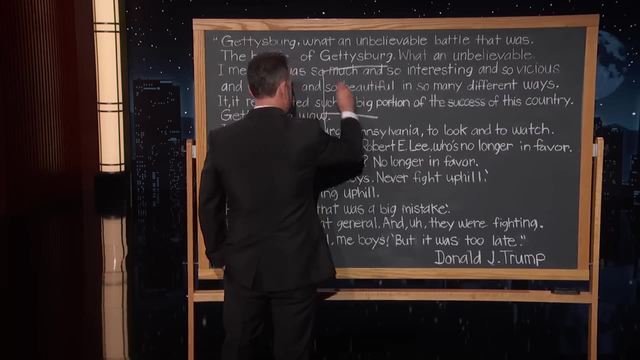 He lost his great general and they were fighting. Never fight uphill me, boys. But it was too late. When you see it written out, it makes a lot more sense. I'm just going to give that a grade NF plus, right. 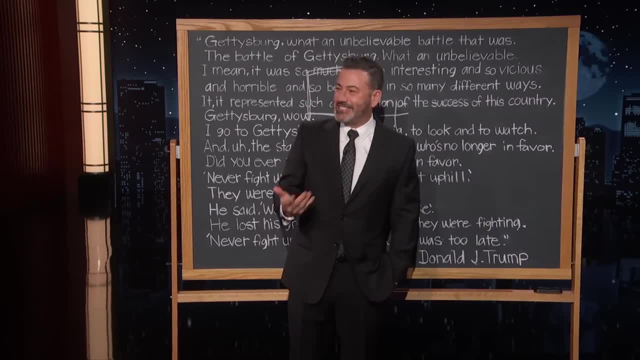 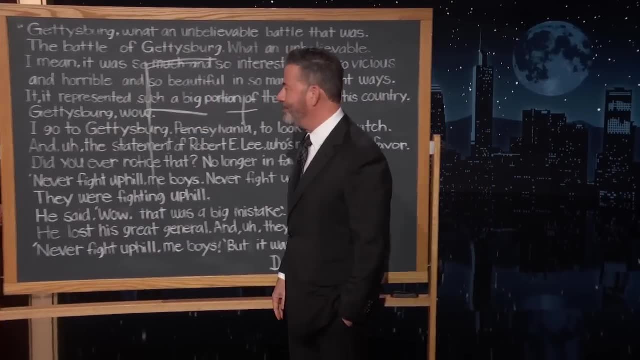 I mean. Robert E Lee said: never fight uphill me boys. Was he a leprechaun or something? You can have that, Guillermo. All right, Never fight uphill me boys And you buy me a me pillow while you're at it. 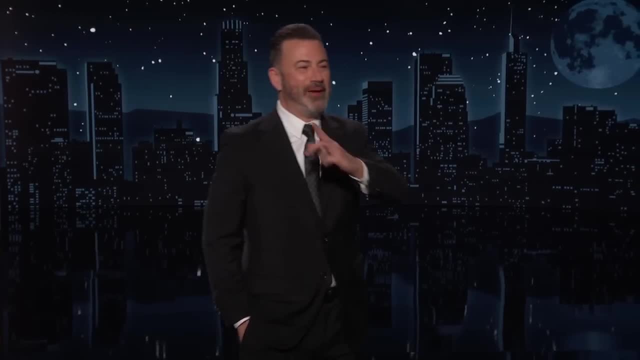 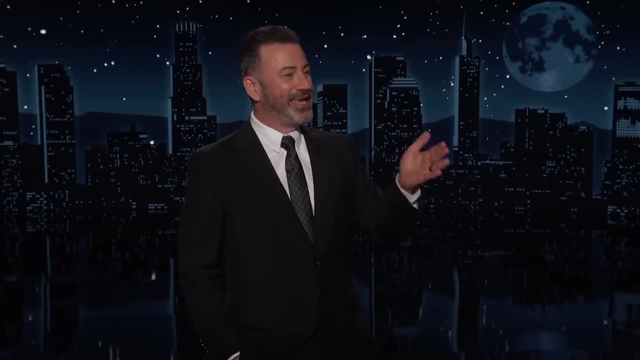 That was something special. That was like get that man on Drunk History, will you? And, by the way, Schnecksville, where he's speaking, is two, Two and a half hours away from Gettysburg. He wasn't even at Gettysburg when he's. 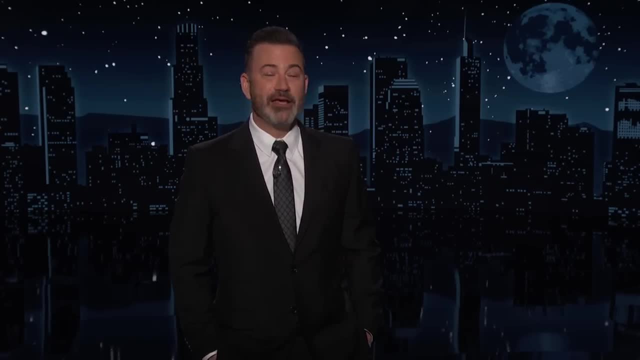 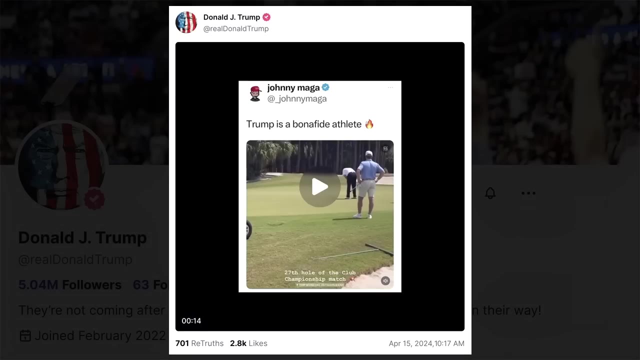 But don't tell Schnecky Green, he wasn't there, He's all over the place. 13 minutes after his trial started today, he posted not one, not two, but three separate videos boasting about winning his golf tournament at his country club. 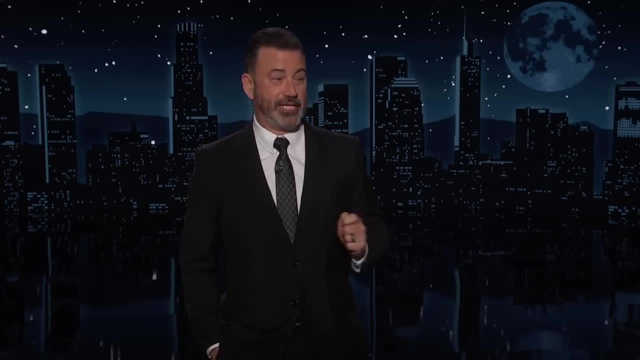 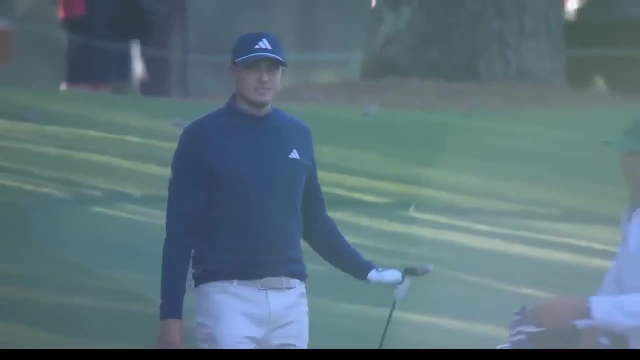 Unhappy. Guillermo did not qualify for the Masters this weekend. He was cheated out of that too, which is a shame, because I think he got a shout-out from Jim Nance. Got away with a poor swing there, He knows it. 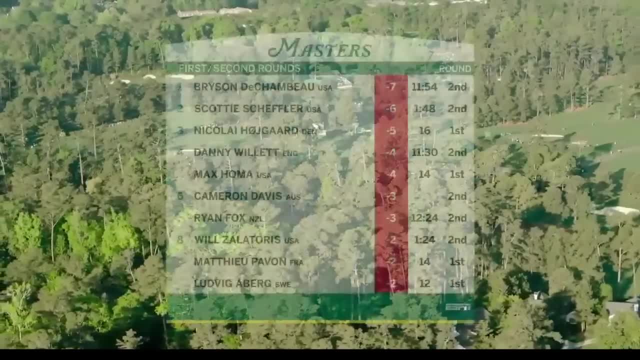 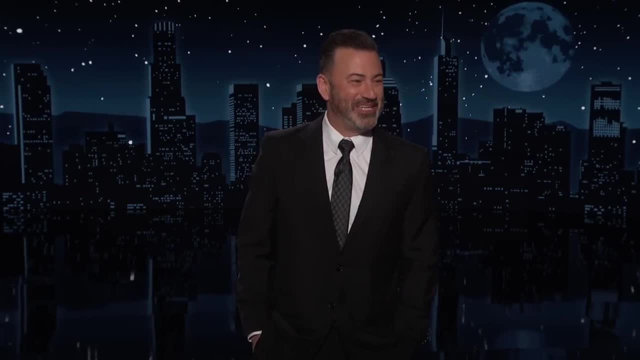 He also knows there's a ticklish little pitch coming up. I'm pretty sure Jim was saying pitch, but I don't know, maybe not. I don't know It's the kind of talk that could get me to start watching golf. 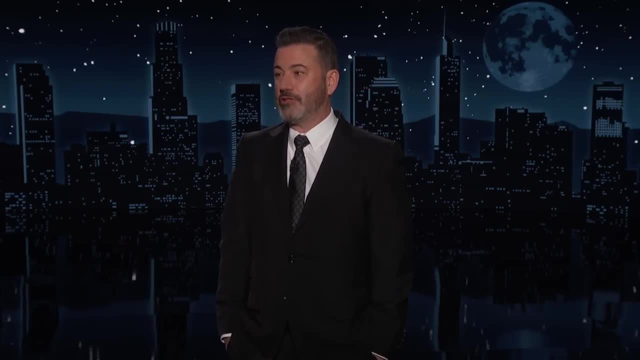 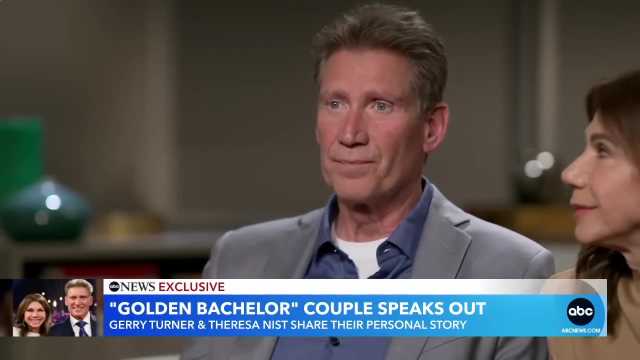 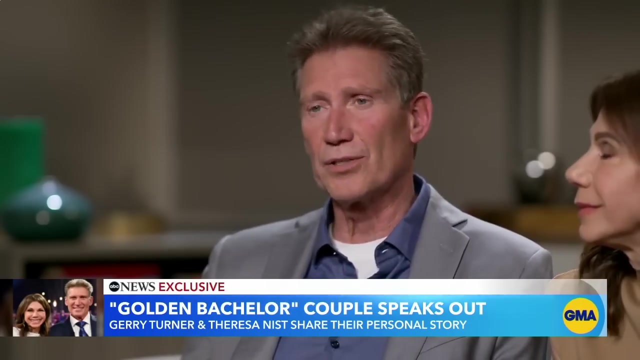 And then we have, maybe the biggest story of the year so far, a bombshell announcement from Gary the golden bachelor and his bride, Teresa and I have had a number of heart-to-heart conversations and we've looked closely at our situation, our living situation and so forth. 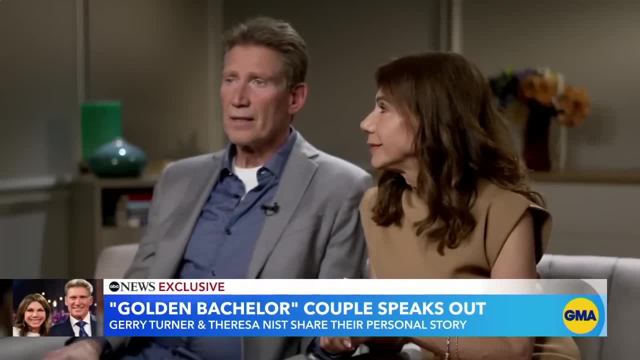 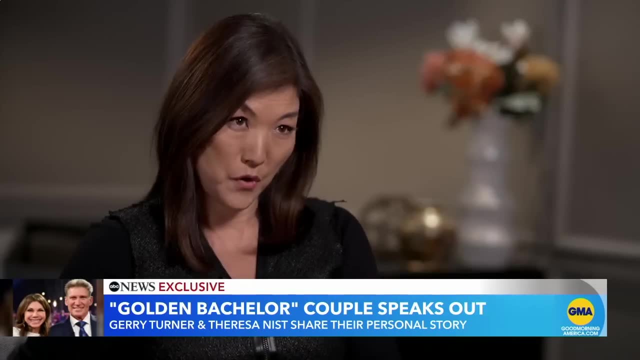 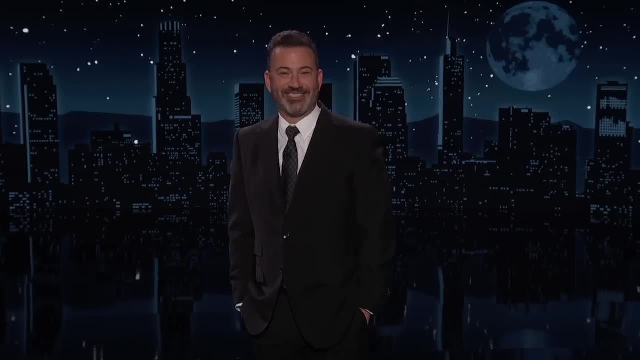 and we've kind of come to the conclusion mutually that it's probably time for us to dissolve our marriage. Get a divorce: Yes, Three months after getting married. Yes, Three months. Gary takes peas longer than that marriage lasted, That's three. 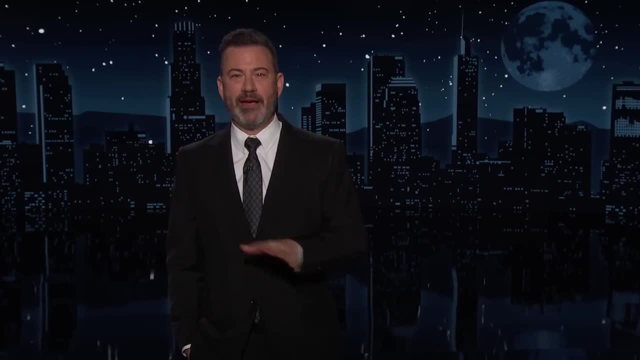 I think there should be a law, or at least an FCC rule that says: if you get married on TV, you have to get divorced. You have to get divorced. You have to get divorced on TV too. I see your rings, Yes. 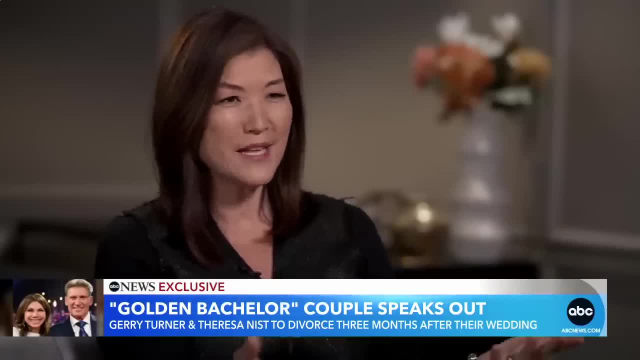 Will you have to give your rings back? Do you give the dress back? How does that work? Oh, I think that's the rule. I think I have to give this ring back. Sad to say, But you know what? We don't have to give back the memories. 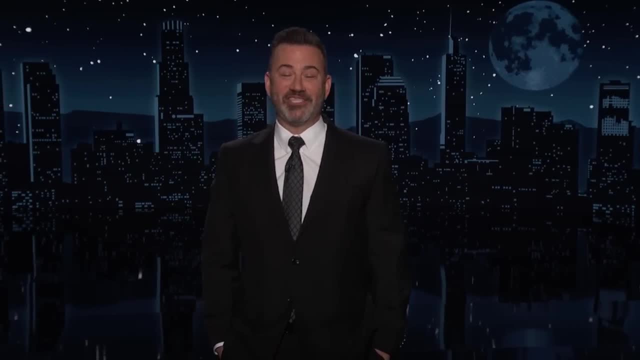 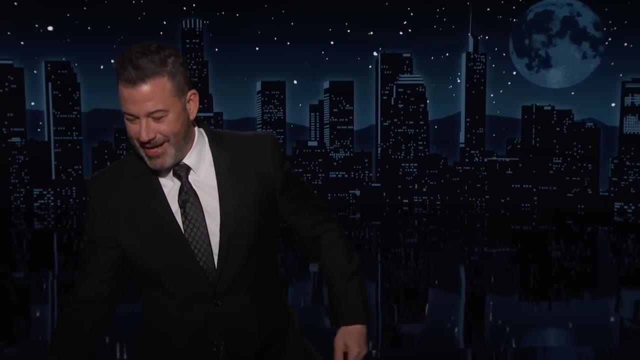 Nice spin, Gary. I see how. Actually, I checked with ABC Legal and you do have to give the memories back. The timing is particularly good because this is Thank you. This is from Emmy Magazine. It's this week's issue. 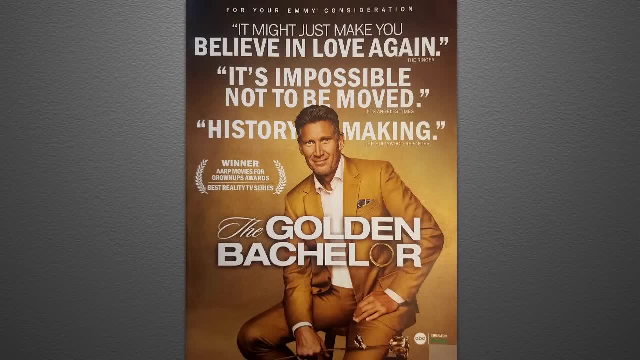 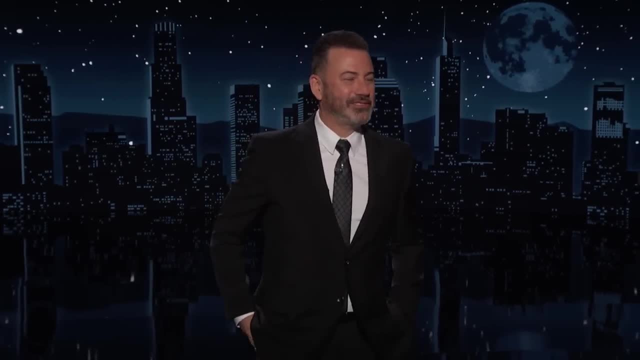 There's an ad for the show. There's an ad for the show that says it might just make you believe in love again, Or not, I guess. So I guess Gary and Teresa won't be filing a joint tax return this year. You know, today is Tax Day. 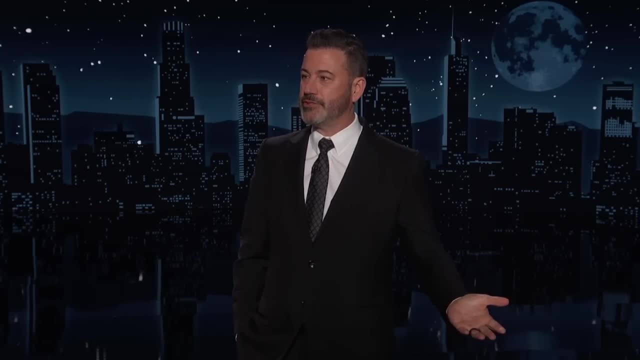 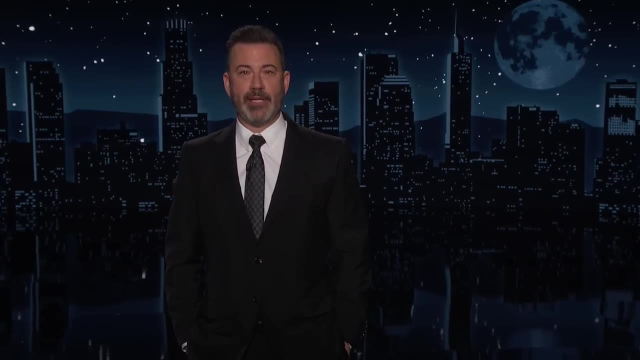 I hope you're aware of that. which is The bad news is: taxes are due. The good news is: starting tomorrow, all our accountants finally have time to hang out again, which will be fun. The deadline to file is at midnight tonight. 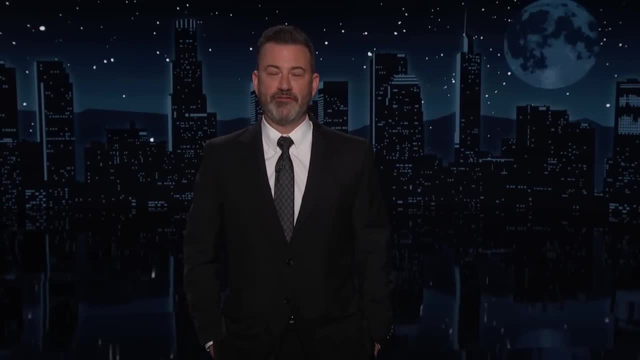 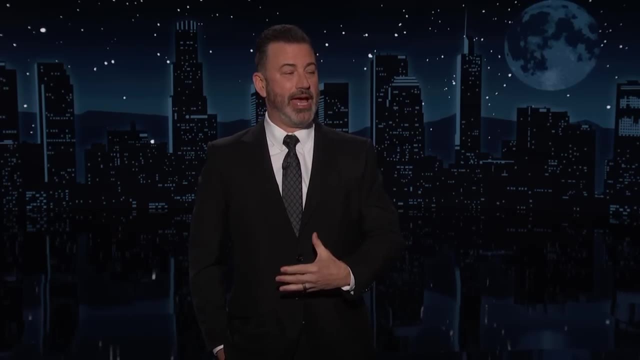 and so we still got around 15 minutes, I think, to squeeze in a few more write-offs. We have a lot of. We have a lot of weird costumes and props that didn't quite make it onto the air this year, And with that said,